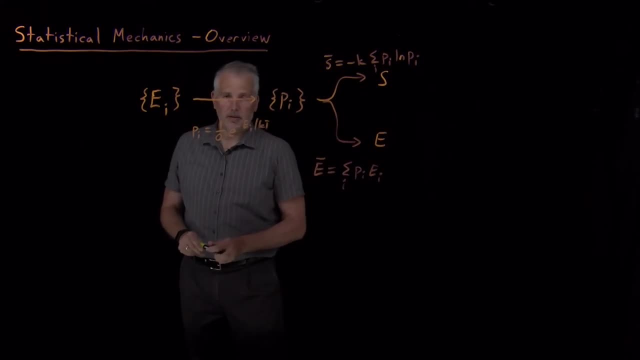 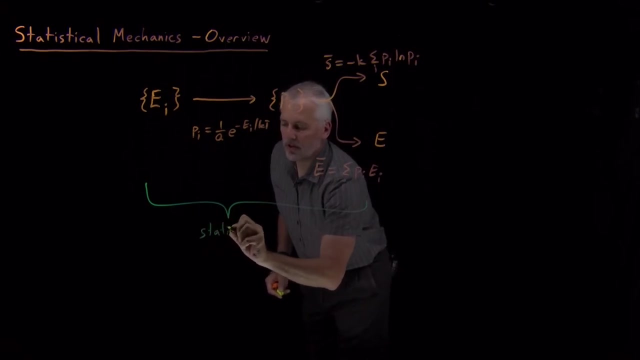 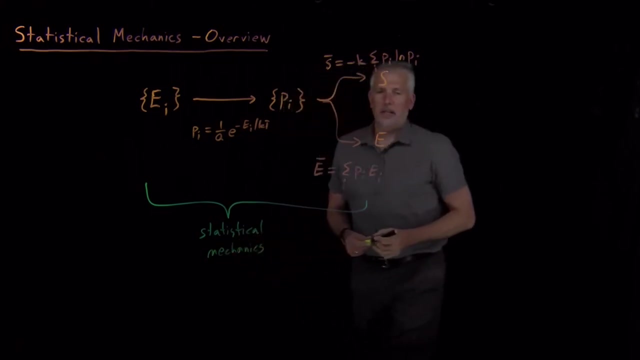 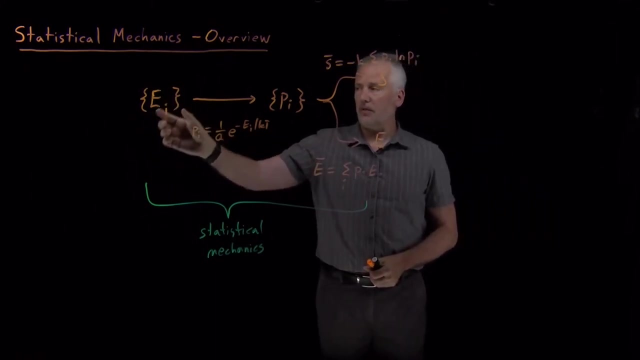 This collection of techniques, equations, is essentially what we refer to when we talk about statistical mechanics, And the whole goal of statistical mechanics is to be able to stop talking about individual, microscopic properties of the system, the individual energies and which particles have which energies, the microstate of the system, and instead be able to talk about collective. 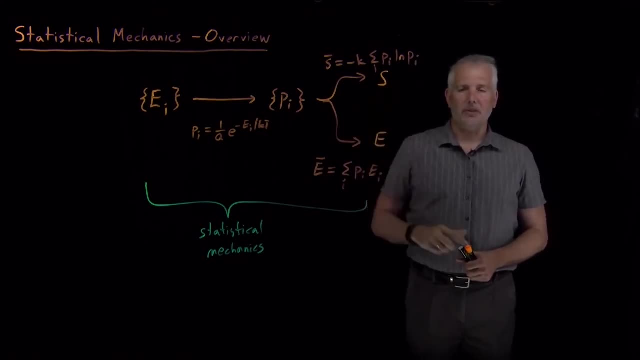 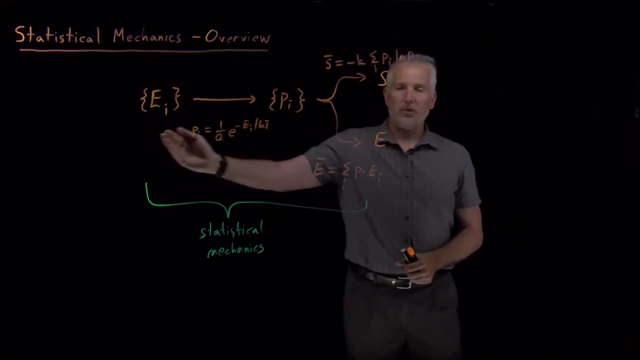 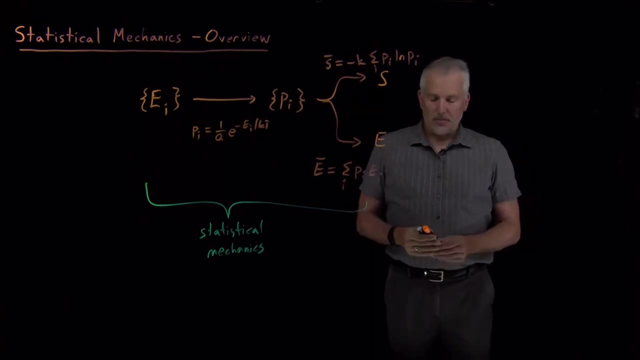 properties of the system, the entropy of the system as a whole, the energy of the system as a whole. Those are things that help us describe macrostates of the system. So statistical mechanics help us move from microstates over to macrostates. Those macrostates, things like the entropy and the energy, those themselves are useful. 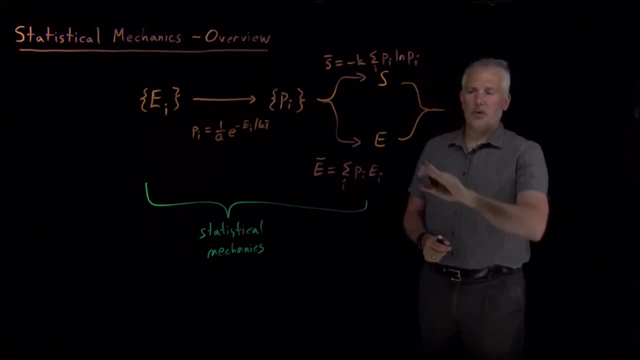 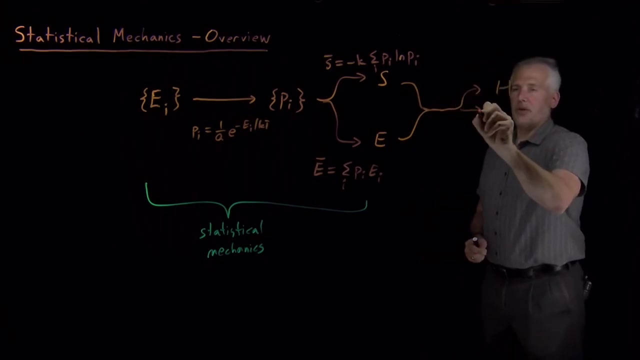 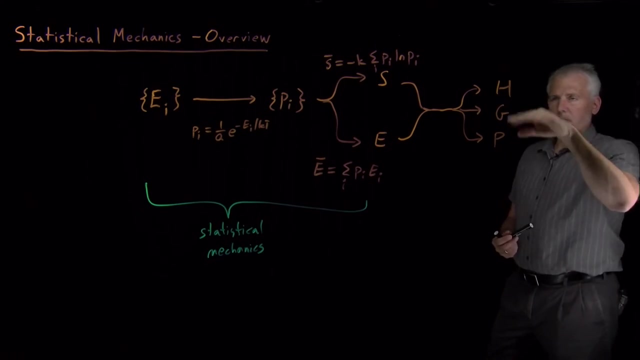 for calculating. Okay, Let's talk about calculating other properties. Once we know something about energy and entropy, we can calculate things like enthalpies or free energies or pressures, other thermodynamic properties. So those are terms that are familiar from earlier chemistry courses, but we'll learn. 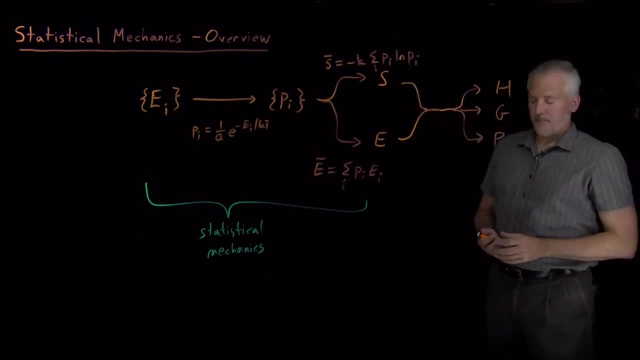 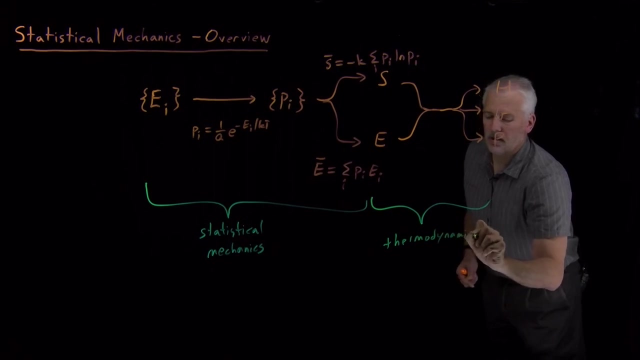 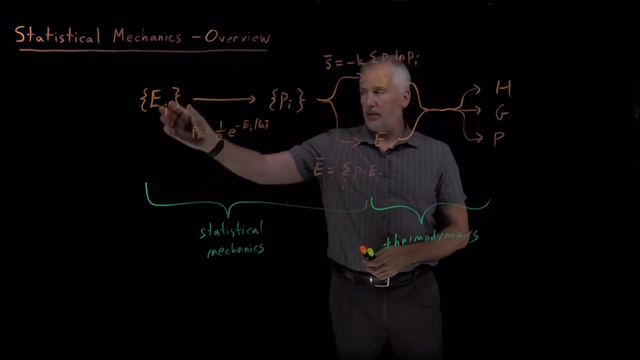 a lot more about how to calculate those from the entropy and the energy. This calculation, The relationship between all these different thermodynamic variables, that's what we're talking about when we're talking about thermodynamics. So, once statistical mechanics has helped us turn microstates and individual and molecule, 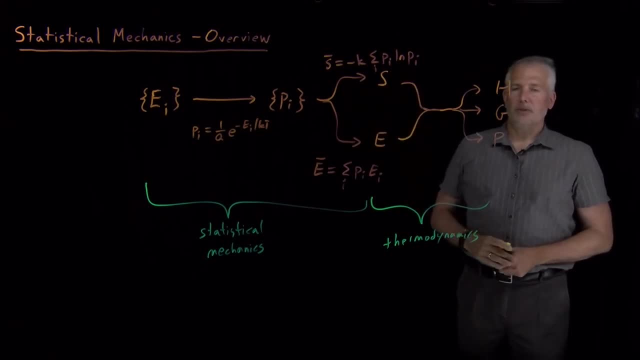 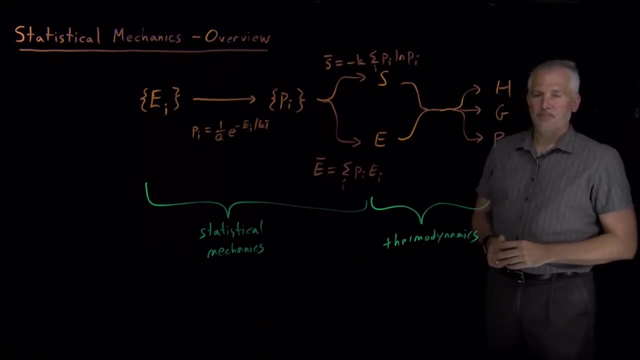 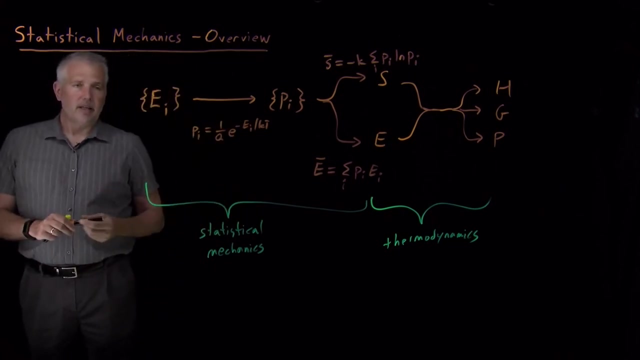 energies into macrostates or descriptions of the system as a whole. the relationships between those properties tell us how to predict other properties of the system using thermodynamics. On the other side, however, before we can do all that Okay, We need to know what the energies are, and it's possible to not just measure but to 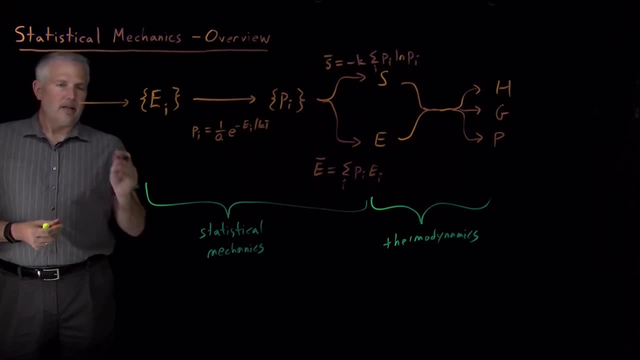 predict or to calculate what those energies are, and that's the next thing. we'll focus on This part of the process: being able to predict what the energy of a molecule or a system is. that's the domain of quantum mechanics, where we'll use different starting points.